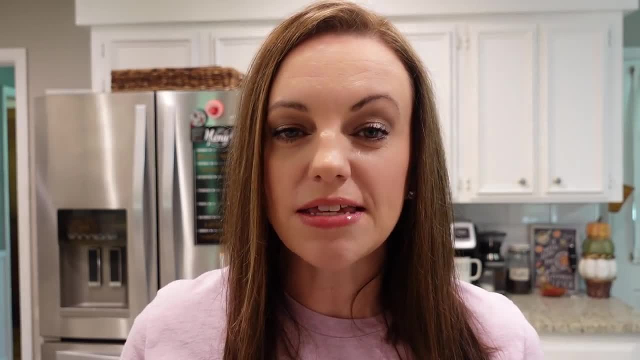 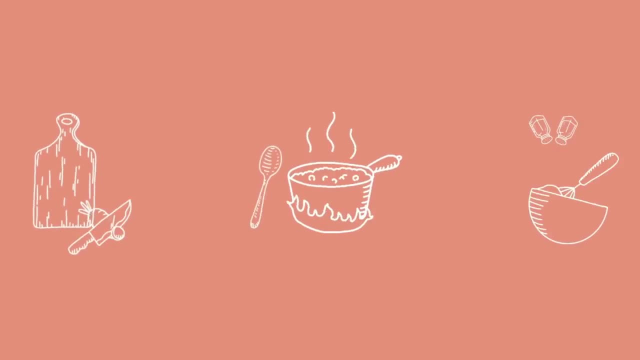 Hey y'all, I'm Mandi, and this is Mandi in the Making. Today, we're going to be making some really cool after-school snacks for your kids and, of course, you're going to love them too. Let's do it. I have a feeling that some of these after-school snack ideas that I'm going to share with you 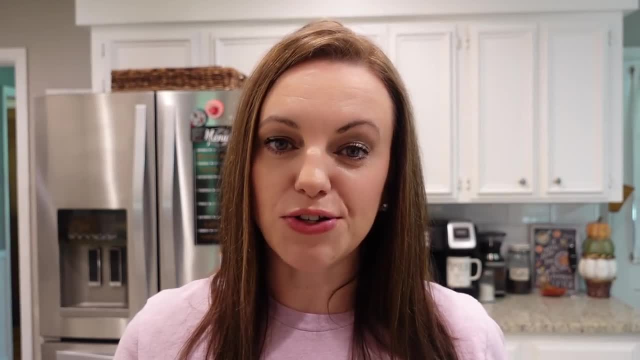 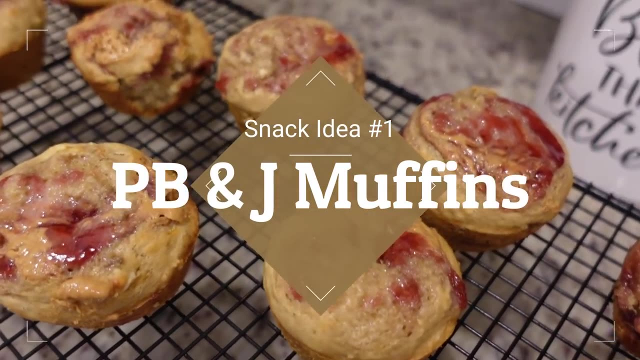 I've got four. they're going to become favorites in your house and your kids are going to request them all the time, and you're probably just going to want them for you too. So the first one we're going to make might be the one I'm the most excited about, and that is peanut butter and 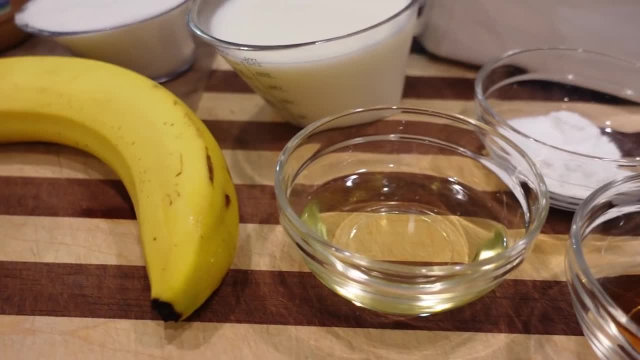 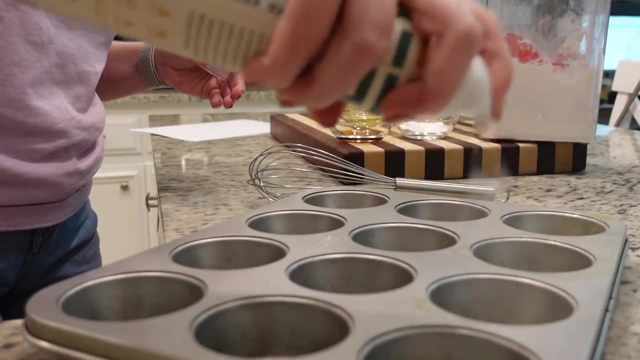 jelly muffins. I mean, who wouldn't love this? My oven is preheated to 375 and I'm just going to spray my muffin tins with a little bit of olive oil so they don't stick. Okay, if you had a banana. 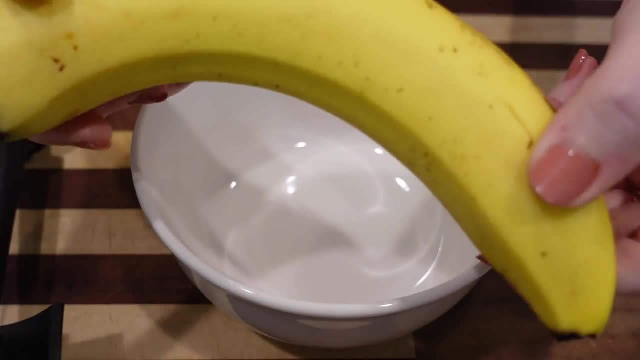 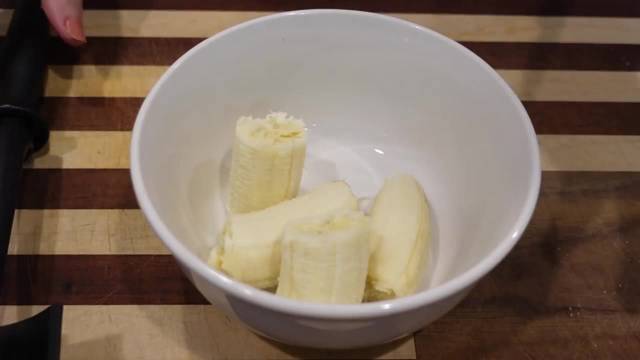 that was more ripe than this. I would definitely do that, but this is the ripest one I have y'all. It's not quite ready to be mashed, but we're going to mash it anyway. You need about a half a cup of mashed banana, and if you've never 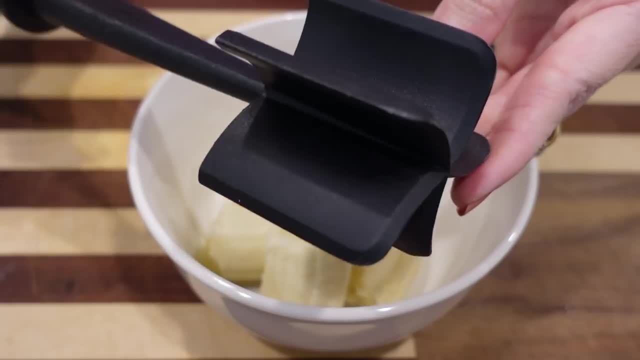 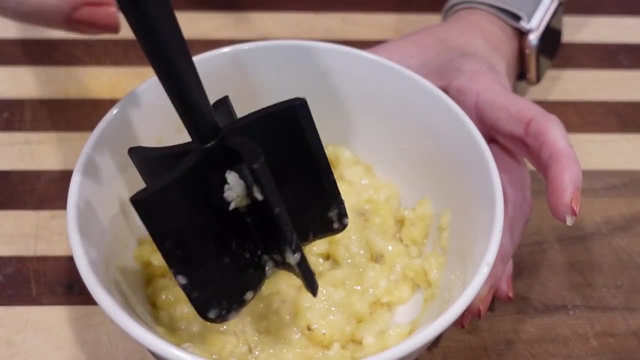 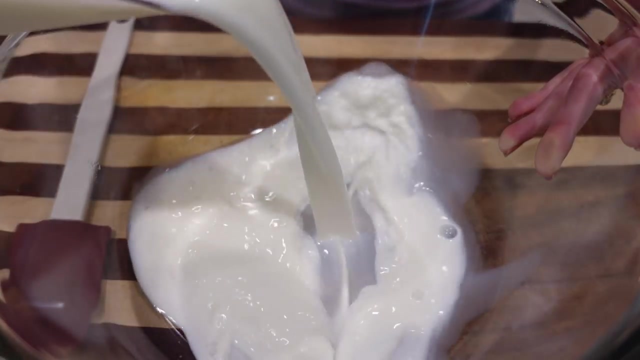 used your mix and chop to chop up or mash up bananas. you're missing out. It really works well. If you don't have a banana, you could always use applesauce in place of this. Okay, so I've got a large bowl here. We're going to start whisking some ingredients together. I 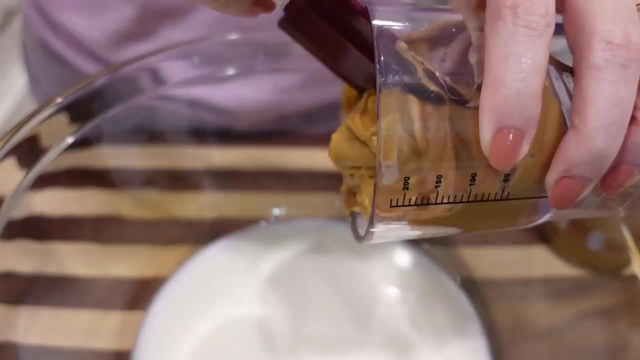 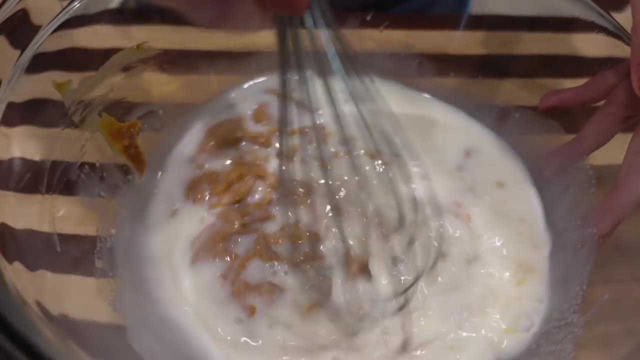 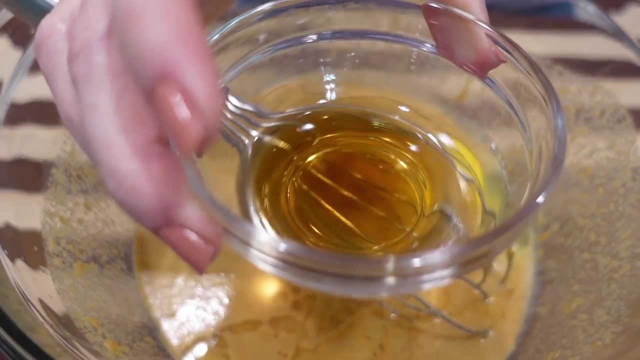 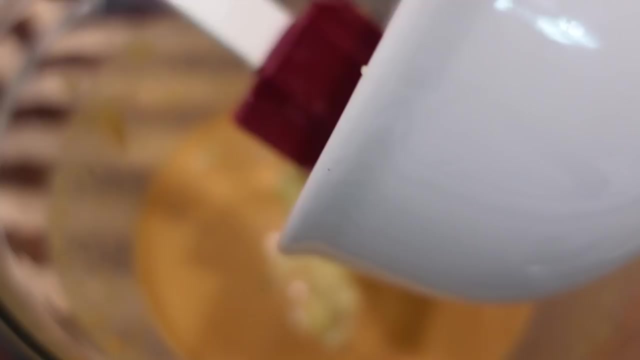 need one cup of milk, a half a cup of creamy peanut butter and a half a cup of sugar. Now to this we're going to add one egg, two tablespoons of oil and one and a half teaspoons of vanilla. Now we're going to fold in our bananas and we're going to stir it until just smooth. Now 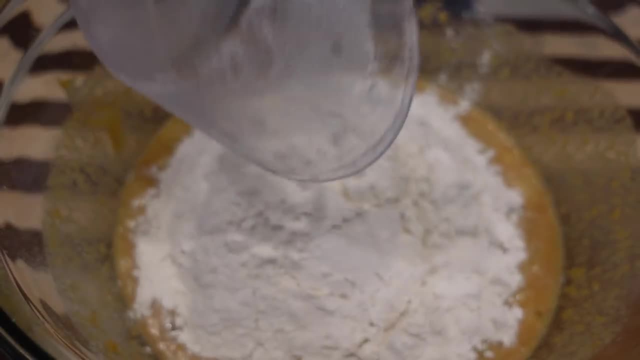 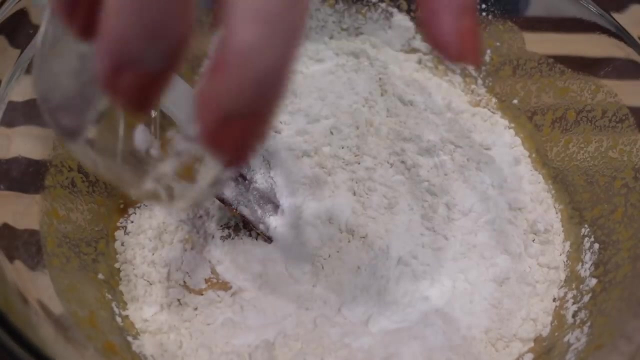 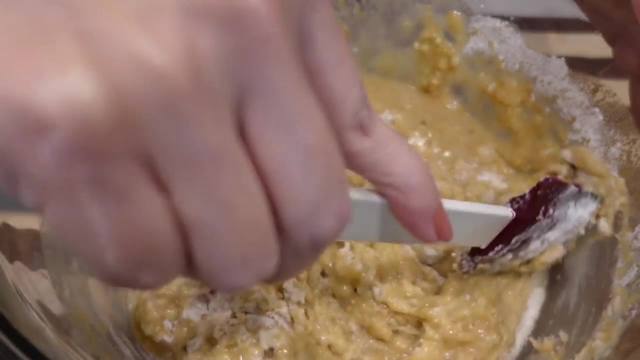 we need one and three-fourths cup of all-purpose flour and, lastly, we're just going to add in one teaspoon of baking soda, two teaspoons of baking powder and three-fourths a teaspoon of baking soda. We're just mixing this until it's combined, and then it will be time to go into the muffin tin. 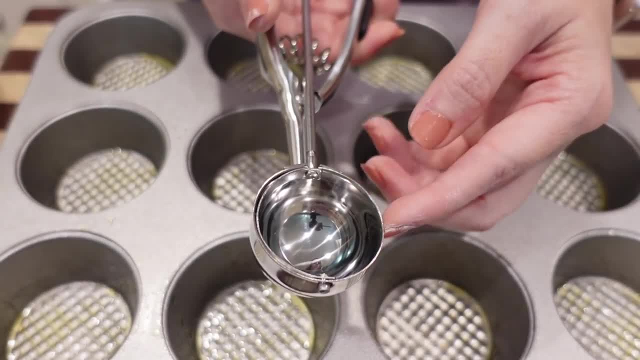 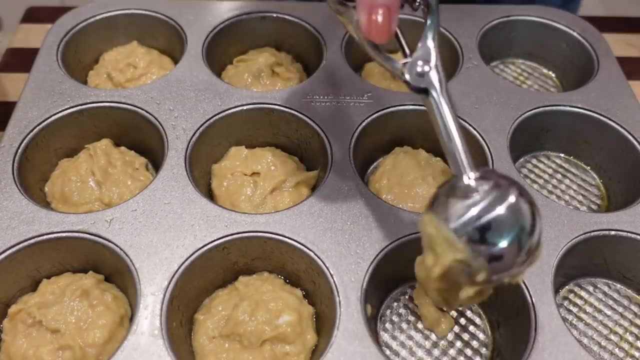 Okay, I've got my little scoop here. If you don't have a scooper, you're just going to put about one and a half tablespoons into each one, so you're not going to fill them up Now. we're going to put about a teaspoon of jam in there. 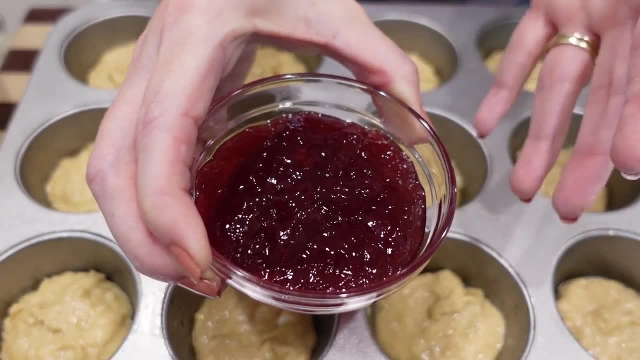 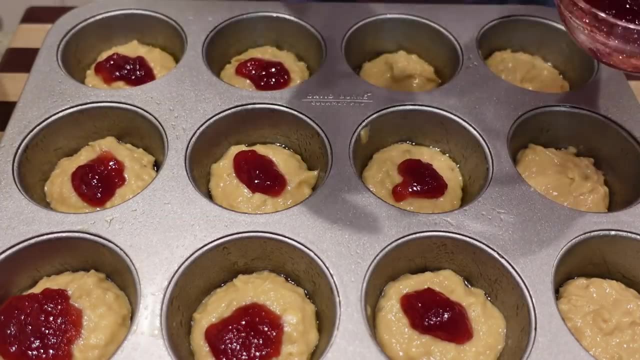 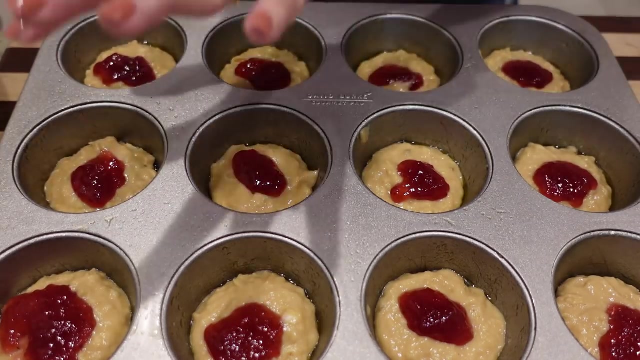 In the middle of each one. I'm using strawberry, which is what the recipe calls for, but you can use whatever jelly jam that you want. Okay, I got a little excited with that first one and overfilled it, but it'll be okay. Now we're just going to cover these with the remaining batter. 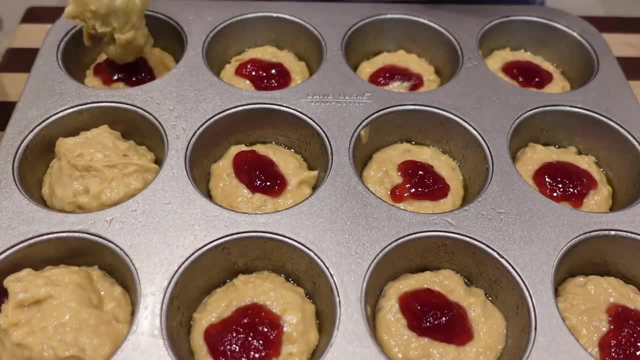 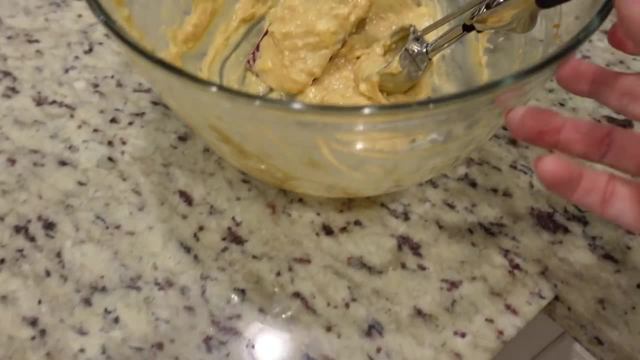 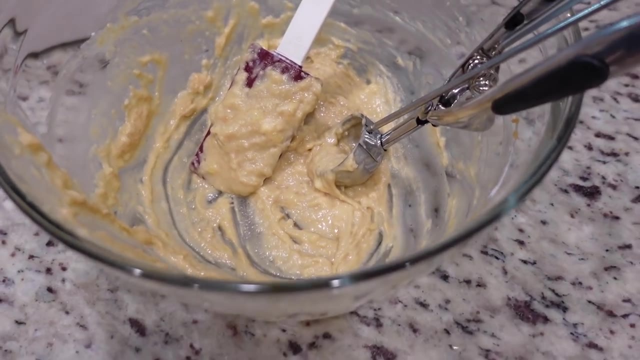 so another scoop on top of each one. So I was able to fill all of these up and I did have just a little bit of jam left over. I was being kind of like careful when I first started because I was scared I would run out. but you won't run out. just a heads up Now to make them look and taste, just a. 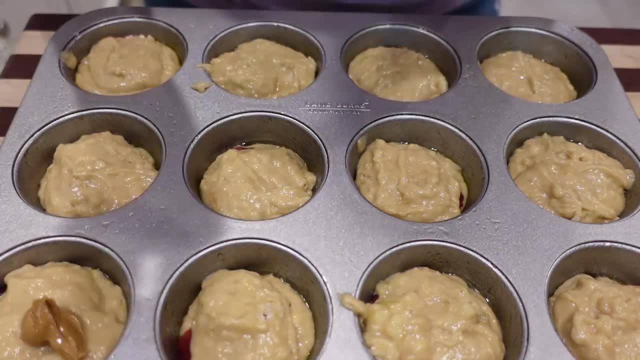 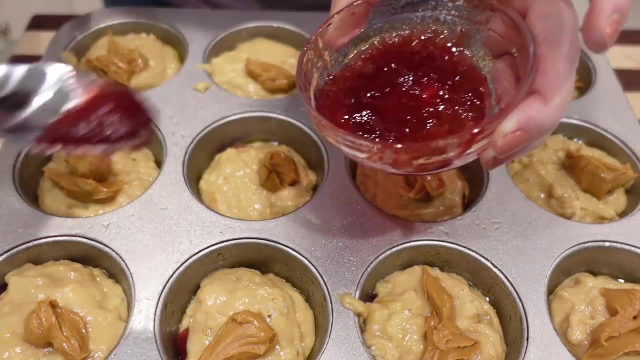 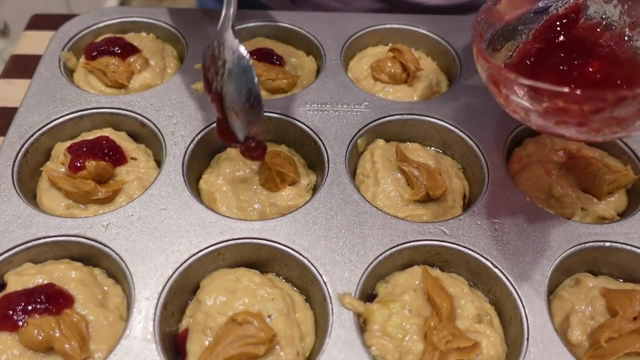 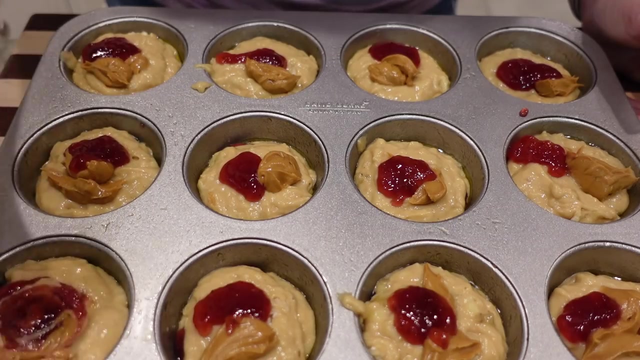 little bit better. we're going to add about a teaspoon of peanut butter on top of each one and about another teaspoon of jam, and then we're going to swirl the two together. I'm just going to use a little toothpick And just kind of swirl these on top. 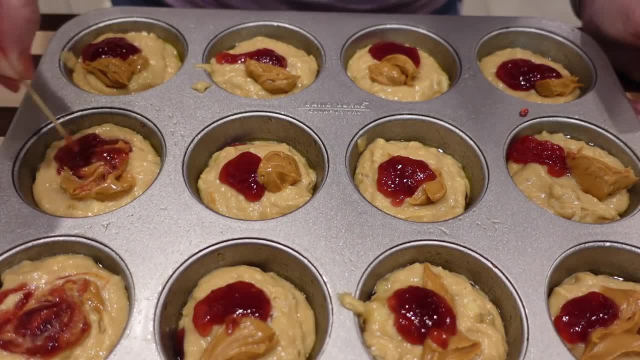 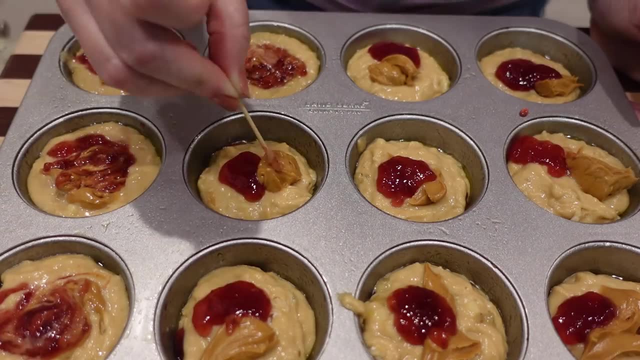 I don't have great swirling skills. in case you can't tell, The peanut butter is kind of hard to swirl because it's kind of stiff, but we're going to make it work. Okay, these are done. They're going to go in the oven at 375 for 15 minutes or until a toothpick comes out clean. 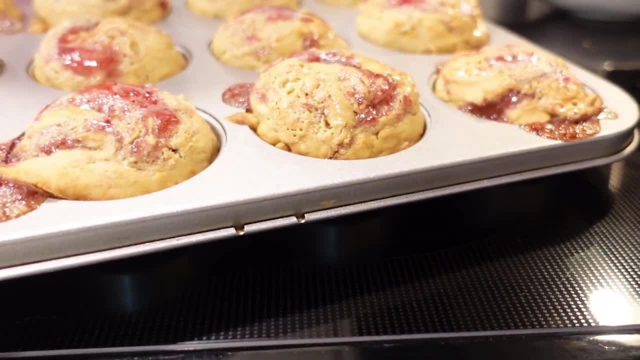 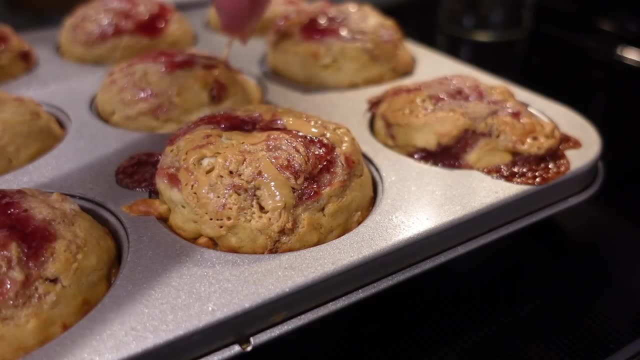 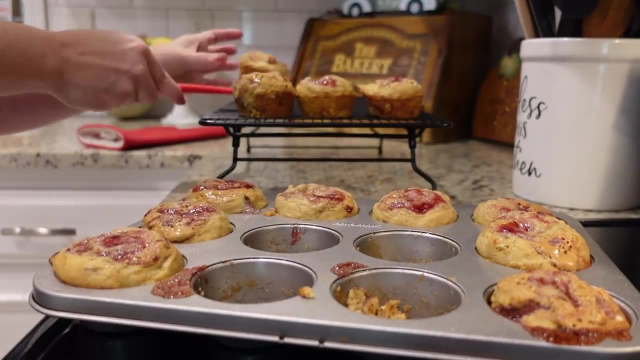 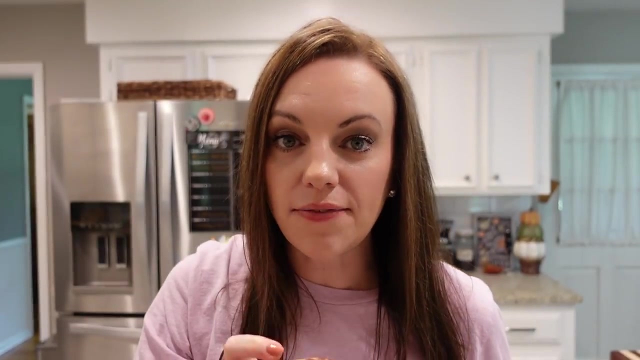 They're going to come out pretty nice and fixed, So okay. so these have cooled. I've already taken one to Steven and he said they're very peanut buttery. They smell like. As soon as I took them out of the oven they smelled like peanuts and I just gotta get them out of the oven. 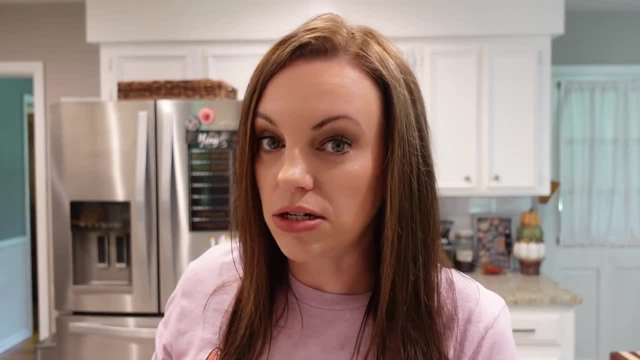 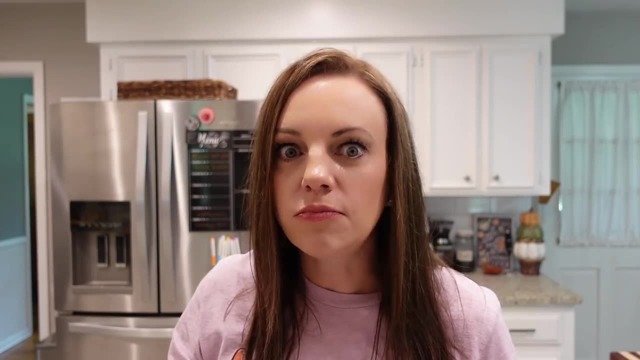 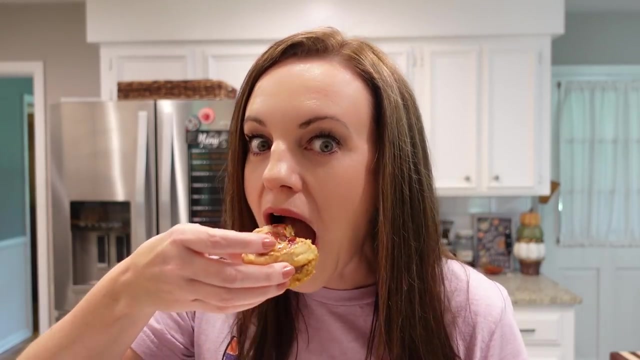 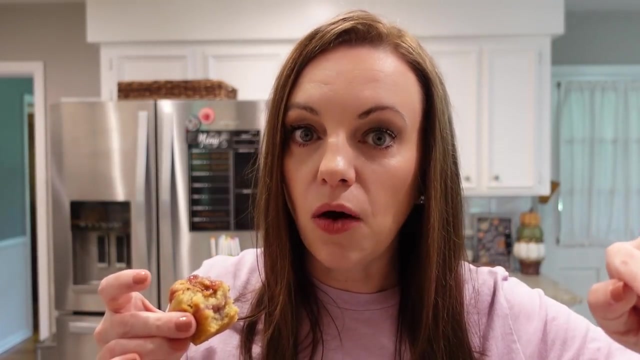 as I took them out of the oven, Stephen wasn't even in the kitchen and he said: I smell peanut butter, So let's give it a try. I mean, that's like a peanut butter and jelly sandwich, but better. Wow, One of these and a small glass of milk. Oh my word, Such a great afterschool snack. 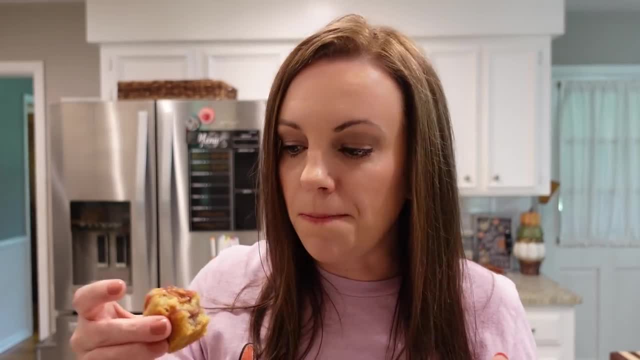 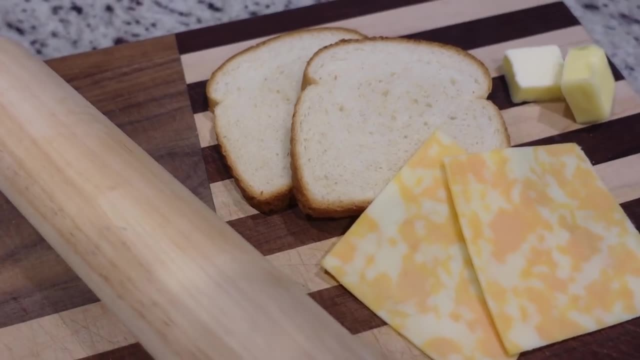 It's definitely rich. You wouldn't want to eat more than one of these, but man, that is good. Our next afterschool snack is a twist on a favorite, and a simple one. It is just grilled cheese roll-ups. You just need cheese, bread and a little bit of butter. You are going. 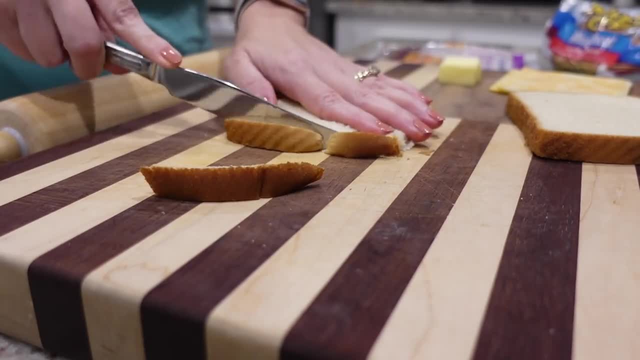 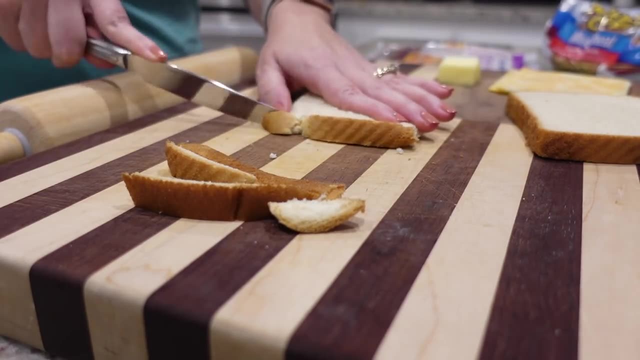 to remove the crusts, which in my case, I was only making two of them, So I just ate the crusts, in all honesty. but you could always dry them out and use them for croutons or something like that. You don't have to waste them. but you're going to remove the crusts and then you're going to flatten. 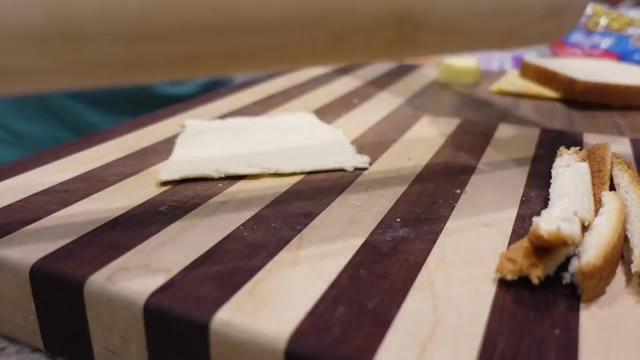 out your piece of bread. I used a rolling pin And then, once it's good and flat, you're just going to grab a piece of cheese and put it on there. Now I used Colby Jack cheese today because that's what I had on hand, but that's a little. 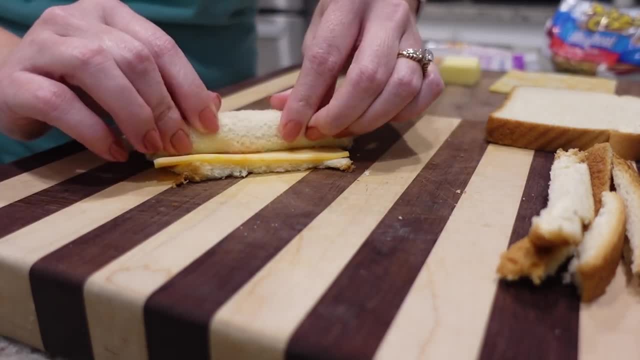 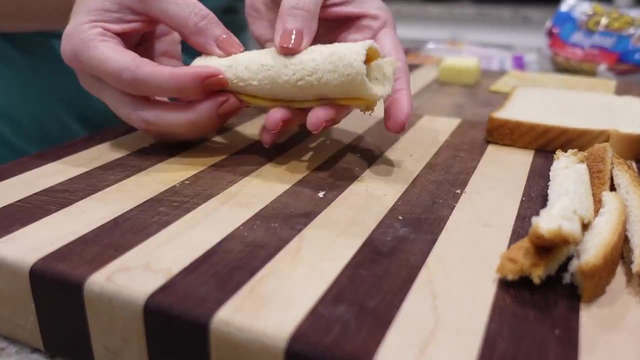 stiffer than something like a Kraft singles, which would be a little bit easier to manipulate. the American cheese Just wanted to throw that out there. I know this is basically just a grilled cheese, but there's something more fun about it being rolled up and being a little bit different. 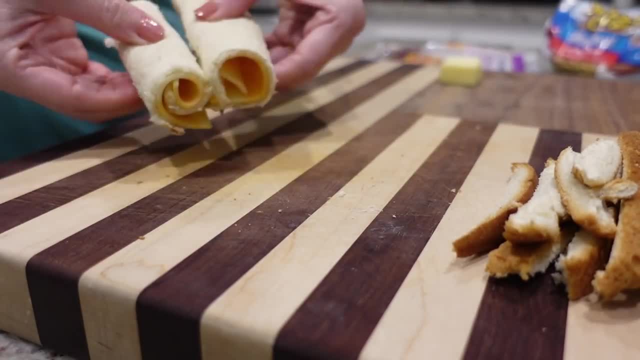 than the usual grilled cheese. So now that we've made these, we're going to take these over to a skillet and I've got it on medium heat. So I'm going to take these over to a skillet and I've got it on medium heat. So I'm going to take these over to a skillet and I've got it on medium heat. 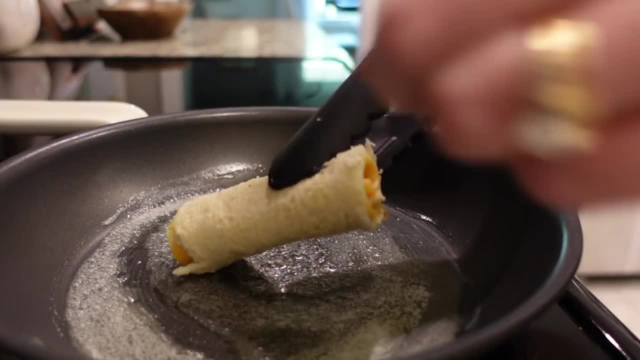 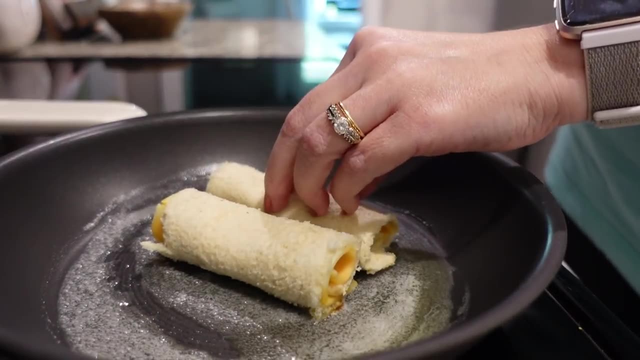 I'm going to add about a tablespoon of butter and let that melt. Then I'm just going to place my roll-ups in the butter and brown them on all sides. You do want to kind of keep an eye on it, because they will try to unroll a little bit on you, especially since I was using that thicker. 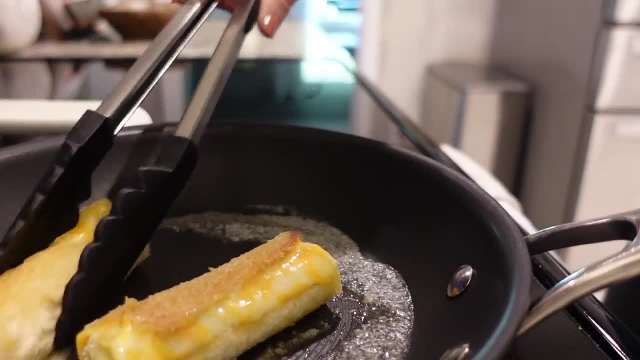 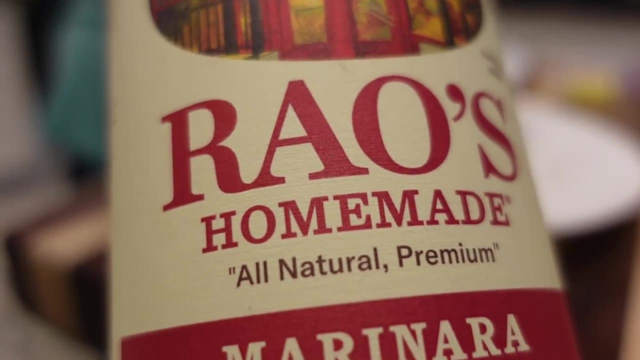 Colby Jack cheese, but it still turned out perfectly. Once they get that good brown color and the cheese is melted, then you know it's done And I'm just serving it with a side of dipping sauce. I'm using the Rao's marinara, which I have recently fallen in love with. It's so good. 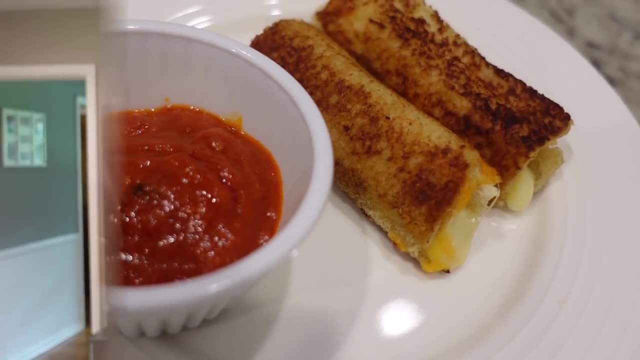 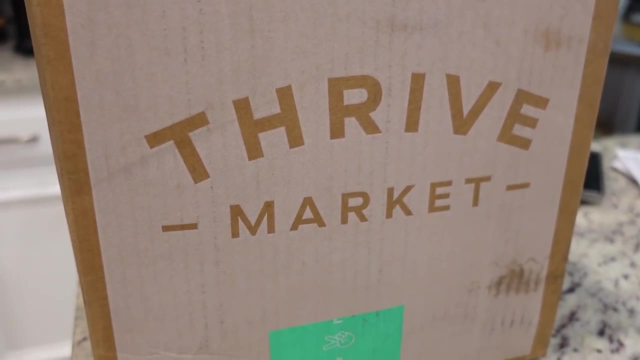 But y'all this was excellent. What a great afterschool snack. Before we get into our next afterschool snack, I did want to thank Thrive Market for sponsoring today's video. I have worked with them several times in the past and, y'all, there's a reason for that. I love their. 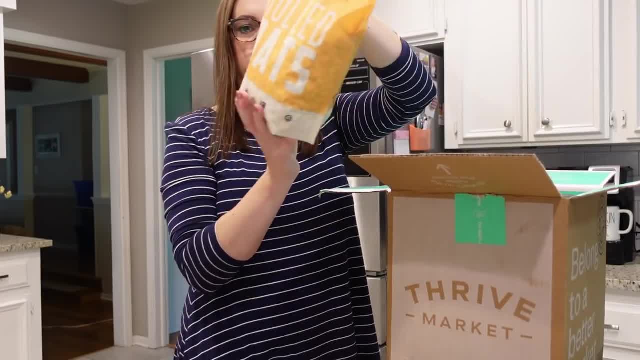 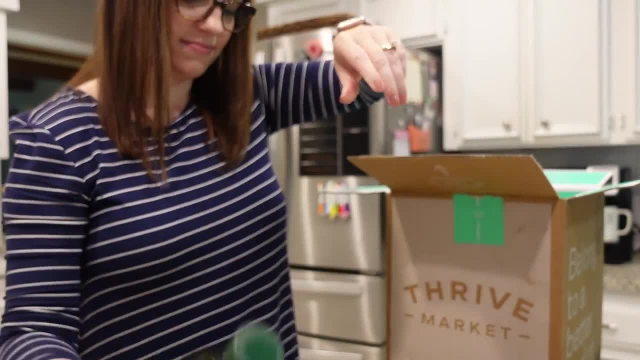 service. So if you already purchase organic products or you are looking to switch to more organic products in the future, this is the place to do it. You're not going to find better prices in the store. So when you join Thrive Market, you're going to enjoy member only prices because 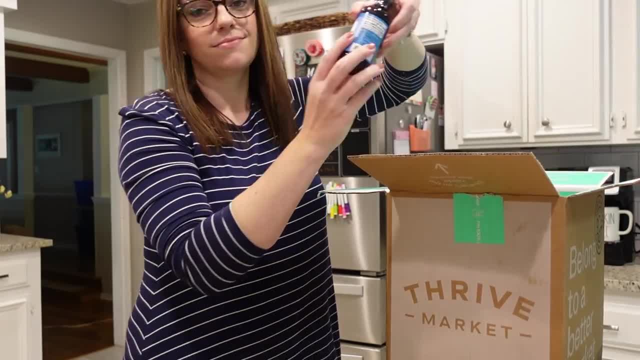 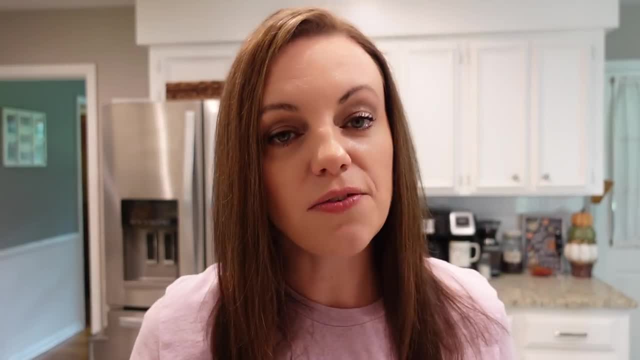 Thrive Market is a place where you can find better prices in the store. So when you join, Thrive Market works directly with some of your favorite organic brands so that you get the highest quality products at the best price. And if you find a better price elsewhere, they will match it A lot. 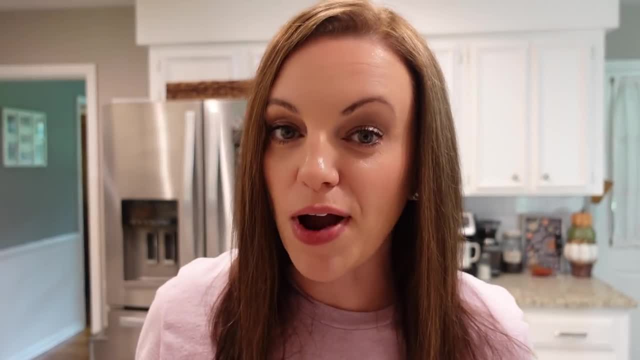 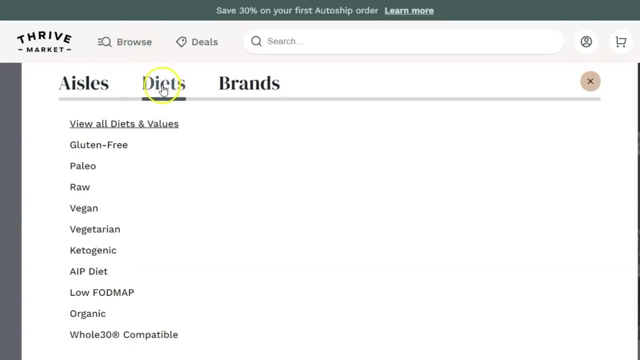 of the products I'm using today to make these afterschool snacks came from Thrive Market, And it's nice to know that these snacks are just a little bit healthier because we're using organic products. If you have a particular diet that you were trying to follow, whether it be vegan or keto, 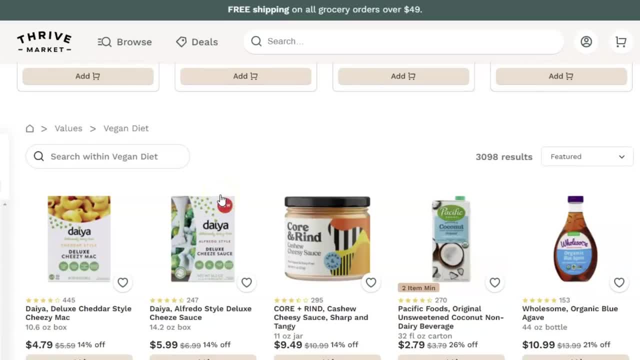 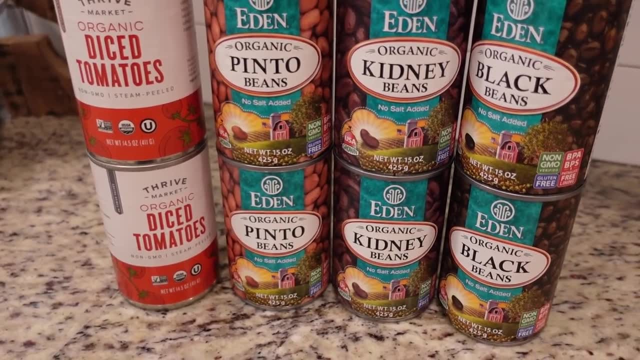 they have an area on the website for you to click on that particular diet And it's going to show you all of the products And it's going to show you all of the products that you're using. So that would fall under that diet for you to choose from. And not only do they have pantry staples like 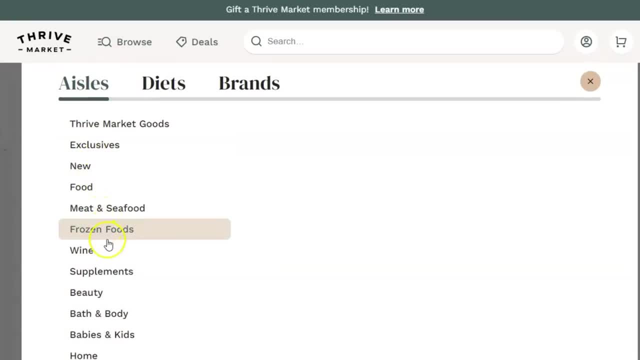 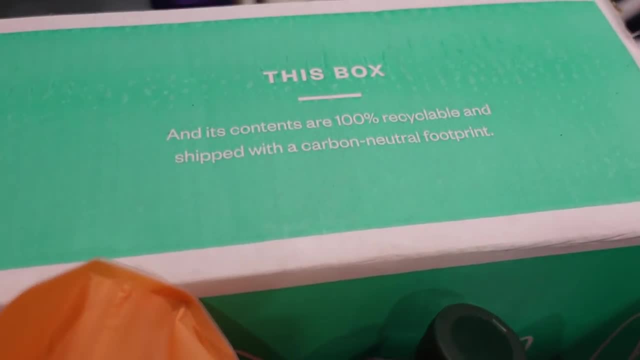 I love, but they also have meat, seafood, non-toxic cleaning products and beauty products. Orders over $49 always ship free And, like I mentioned, you are doing this by being a Thrive member and you can be a member for one month or you can choose to do the entire year We chose. 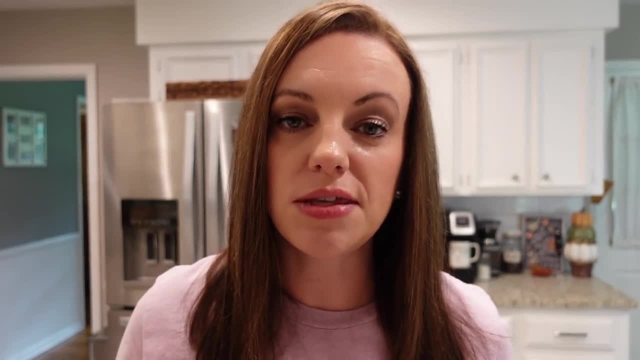 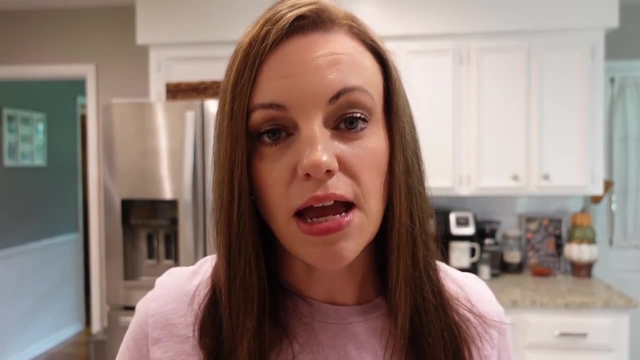 the yearly subscription because it comes out to $5 a month. But if you choose, the monthly membership is $9.95 a month. I really love ordering pantry staples from them. I love getting our honey, our olive oil spray, our extra virgin olive oil. I got their rolled oats. and even some vanilla extract, which I know I'm going to need a lot of these coming up in the holiday season. My advice would be to download the Thrive app And, as you start to run low on things in your pantry, start adding things to your order And, once you hit that $49 threshold, 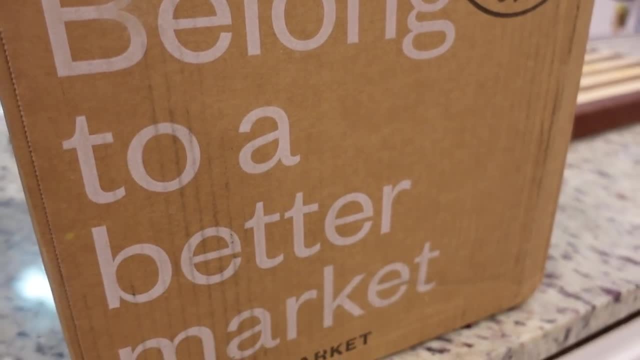 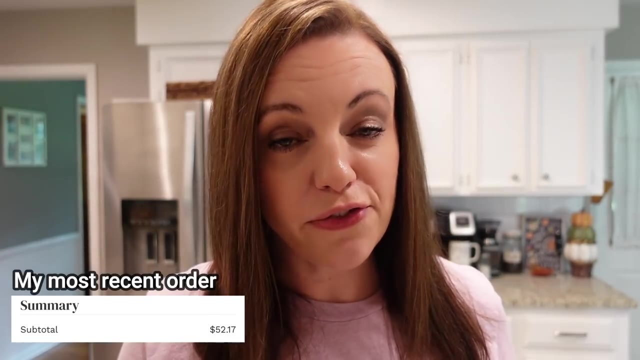 it ships for free. Go ahead and check out and get all of your goods right to your door. I usually create orders And once I get to that $49, $50 range, I go ahead and have it shipped. That way it ships for free. But the great thing is, I can look at the price comparisons and see how. 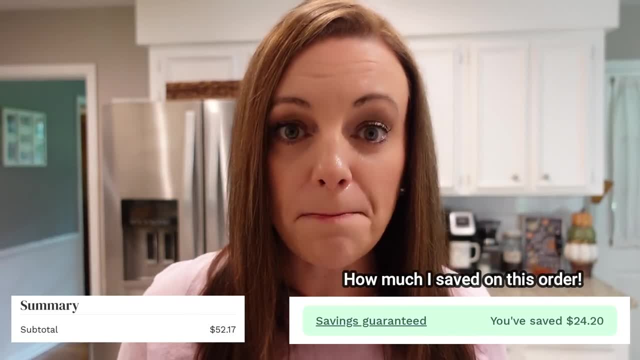 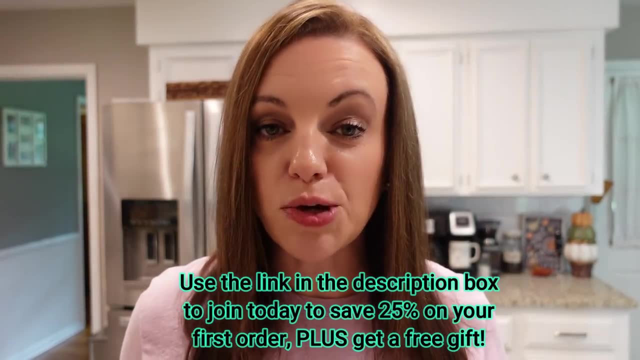 much I saved- And on average I saved $22 to $25 per order- as compared to buying it in store somewhere. So if you are interested, I highly recommend checking them out, And if you'll use the link below and join today, you're going to get 25% off your first order, plus a free gift. 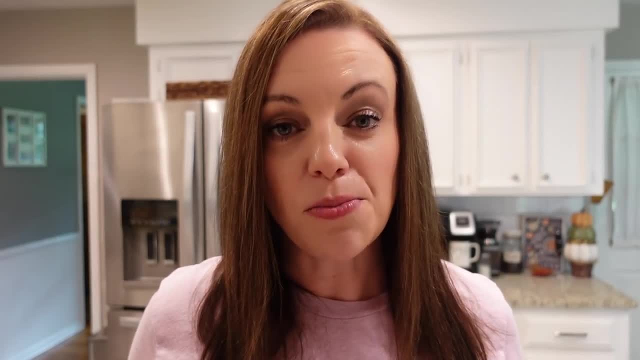 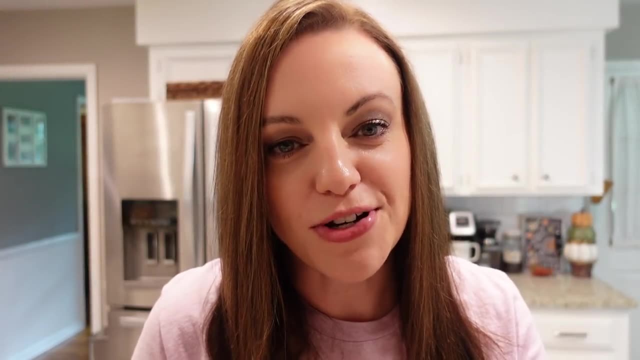 And if you do join today, just know that you're helping out someone in need, because with every paid membership, Thrive gifts a membership to a low-income family. Thanks again to Thrive Market for sponsoring today's video. Let's go back and make some more. 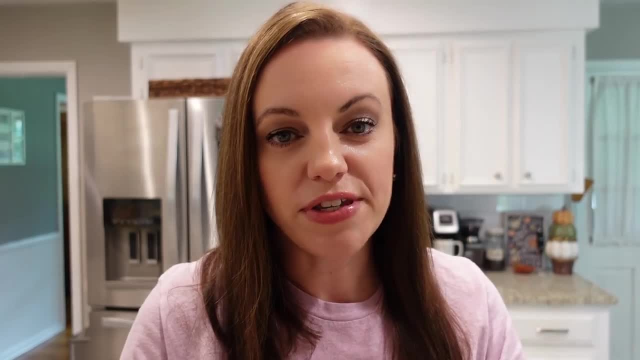 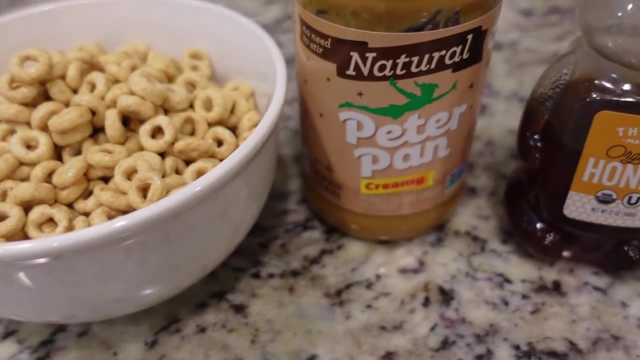 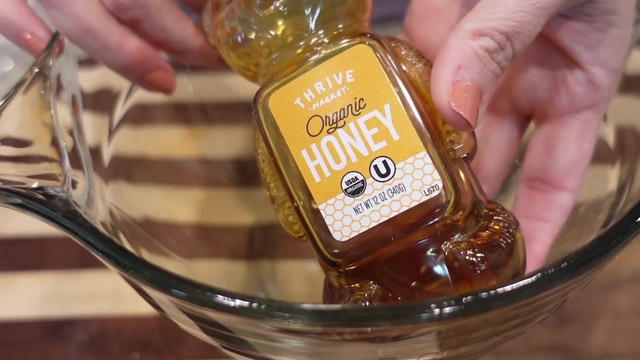 snacks. That rhymed. This next one involves no baking and it's going to take us like five minutes. It's peanut butter cereal bites. Okay, I've got a large glass bowl here. It is microwave safe. I need a fourth a cup of honey. 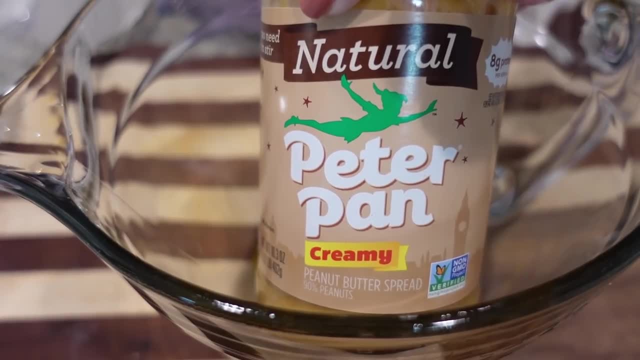 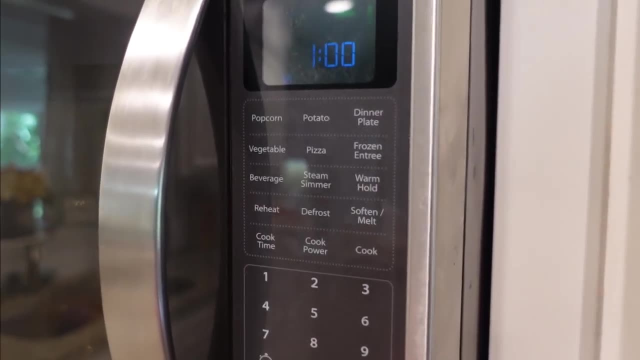 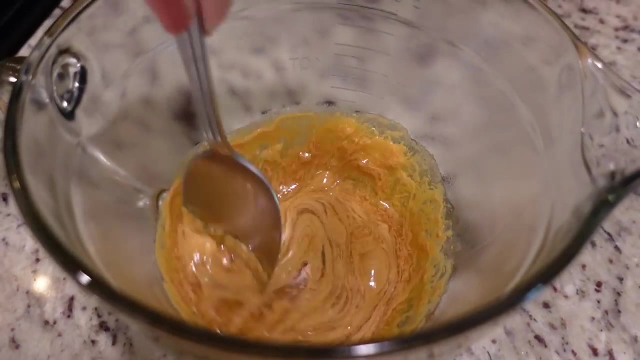 I am cutting this recipe in half and I need a fourth a cup of peanut butter. Okay, we're going to pop this in the microwave for one minute on high. Now we're just going to take it out and stir it And we're going to put it back in the microwave for another 30 seconds. 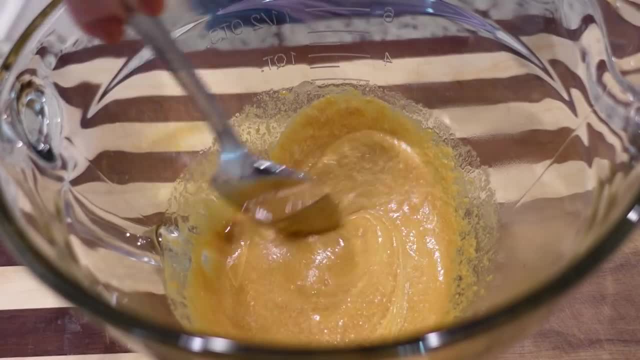 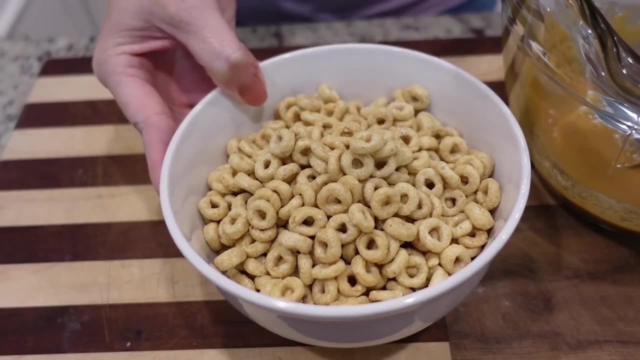 Okay, this is really hot and really well combined. Now let's add in a quarter teaspoon of vanilla extract. Lastly, we're going to add in a quarter teaspoon of vanilla extract. We're going to add in our Cheerios- I have the Honey Nut Cheerios. It does call for plain. 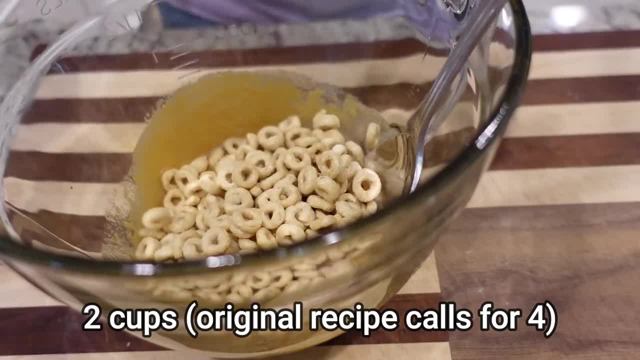 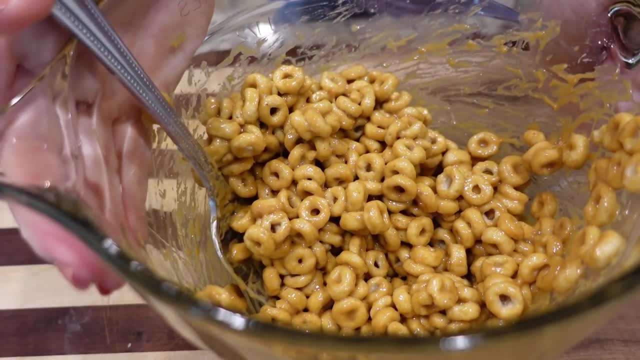 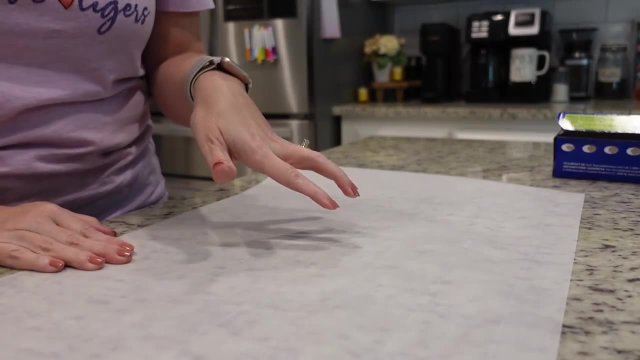 but I didn't want to buy a whole box of plain and not eat them because I don't like plain Cheerios, so I went for the Honey Nut. Okay, let's grab our parchment paper Now. you could put your parchment paper onto a baking sheet so you can move it easier. 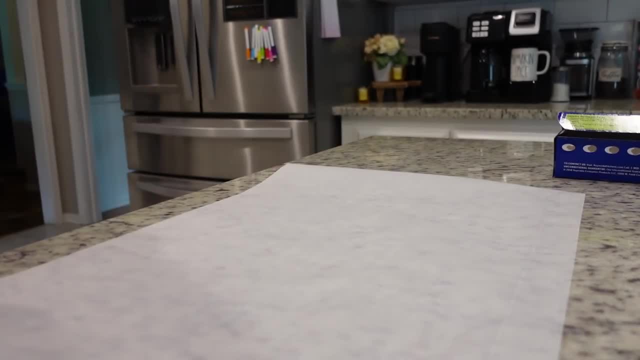 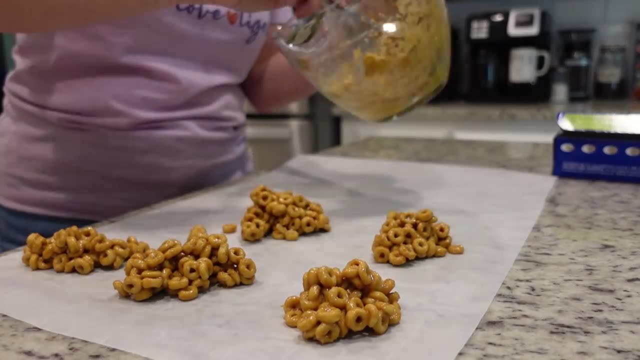 but I don't need to use my countertop anytime soon, so I'm just going to leave it like this. But now we're just going to drop portions of this together Onto the parchment paper and it's going to set for about 30 minutes. 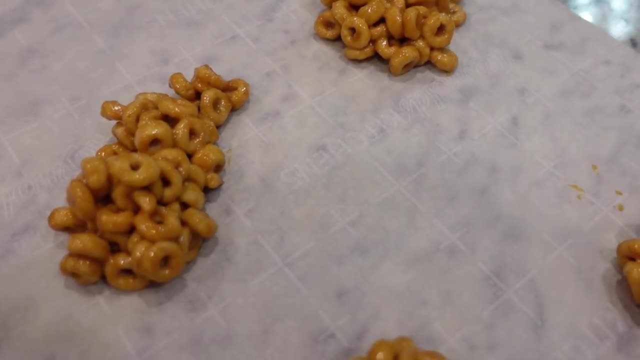 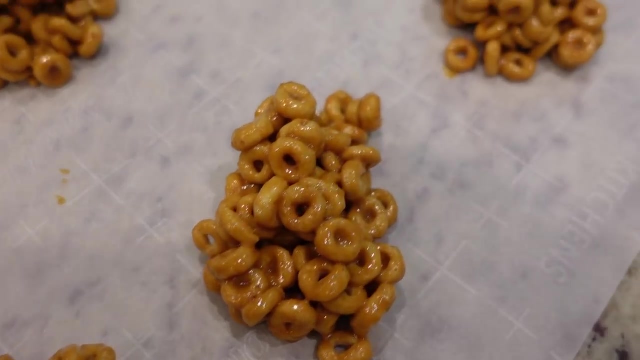 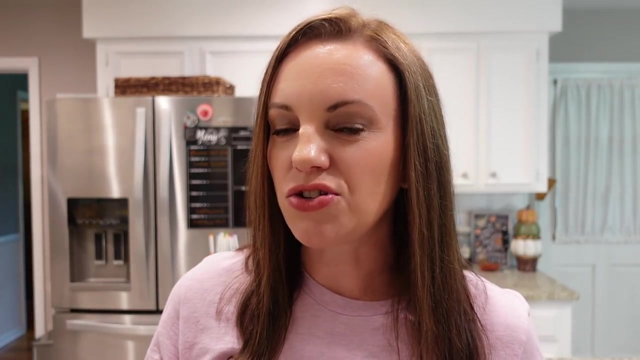 So these are going to take about 30 minutes to set, but it'll take a few hours probably for them to harden, but they smell really good and have a feeling they are going to be very, very tasty. Okay, y'all, it's been a couple of hours, I think. I don't know. I lost track of time. 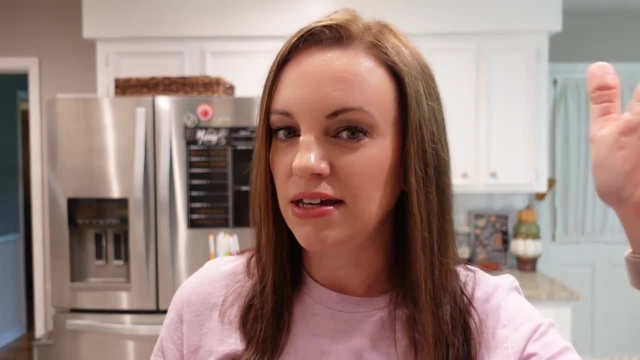 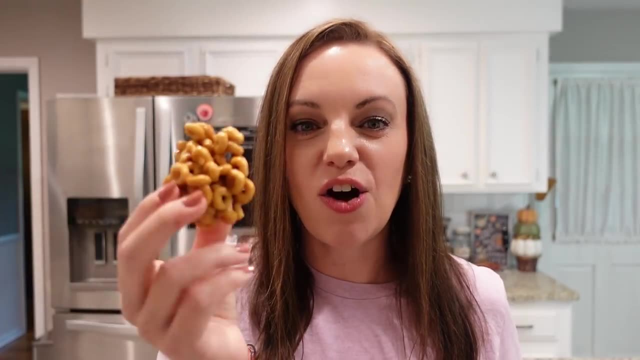 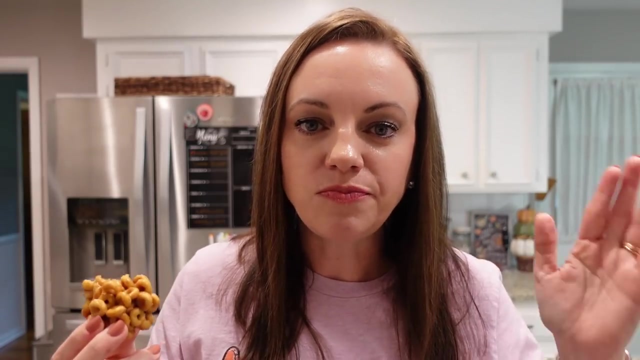 because it's Saturday and college football is on. It's all I want to do is watch college football. It's what I do. Anyway, these have hardened and now it's time to give them a try. I want to keep eating, but let me just tell you these are excellent. 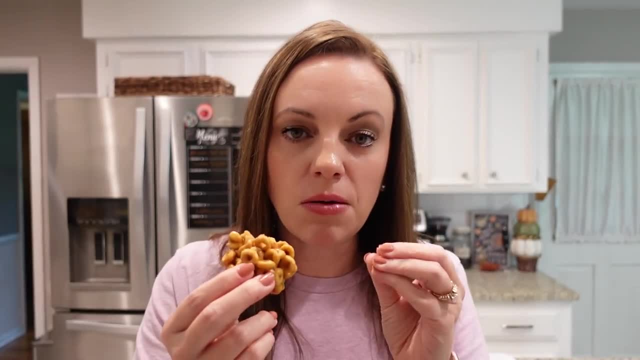 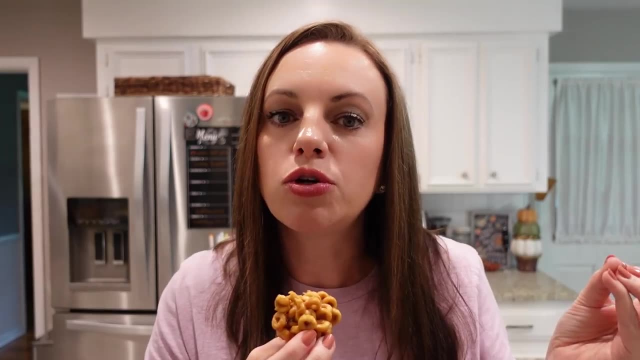 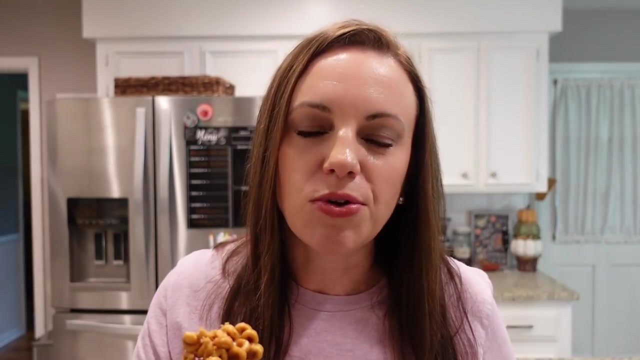 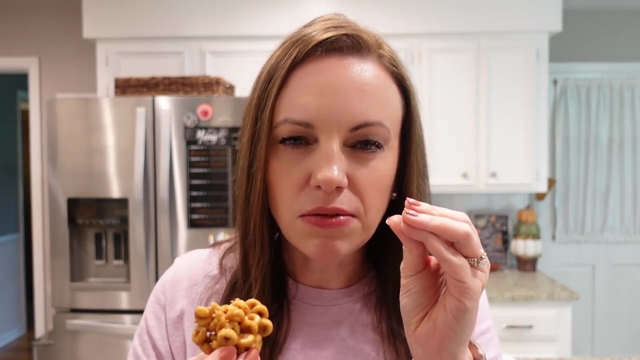 So they still have a good crunch to them. The Cheerios did not get soggy, so that's good. It's kind of like a granola bar, but better in my opinion. I have Y'all tell me what you think. I like chewy granola bars. I'm not a big, really crunchy granola bar. 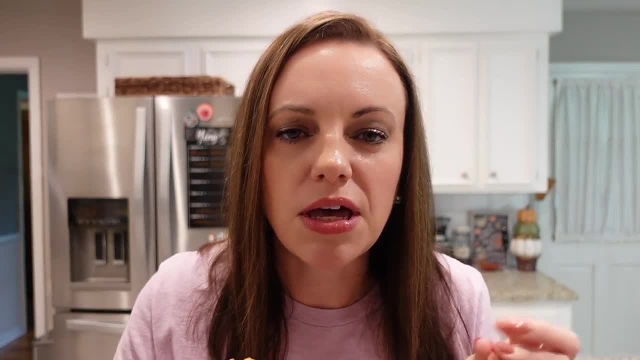 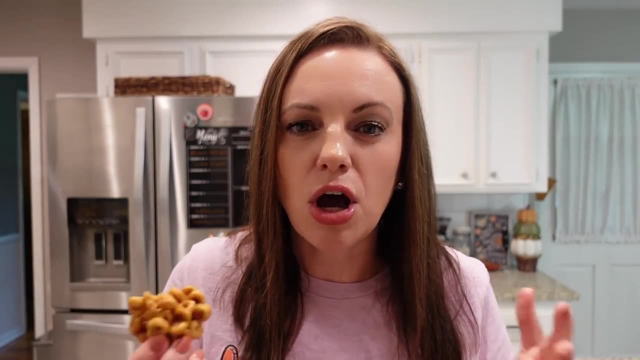 person, but the chewy ones I have a love-hate relationship with because they tend to get stuck in my teeth really badly. So in theory I like granola bars, but if I have an option, I'm going to choose something else. That was a long explanation, just to let you know that these 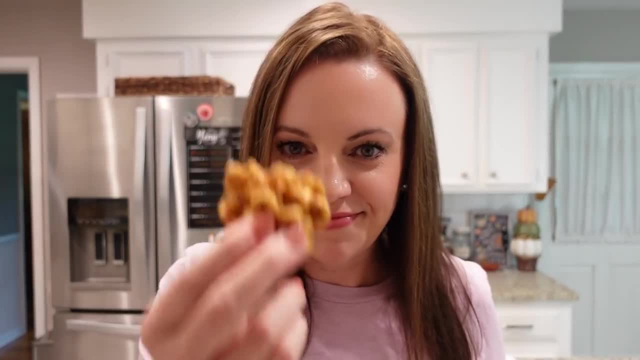 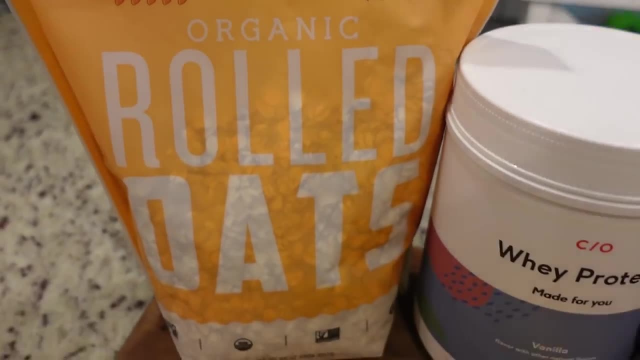 are better than granola bars, but they are, in my opinion. For our last after-school snack idea, we're going to be making no-bake energy balls. These are great to make ahead of time and just store in the freezer and just grab them as you. 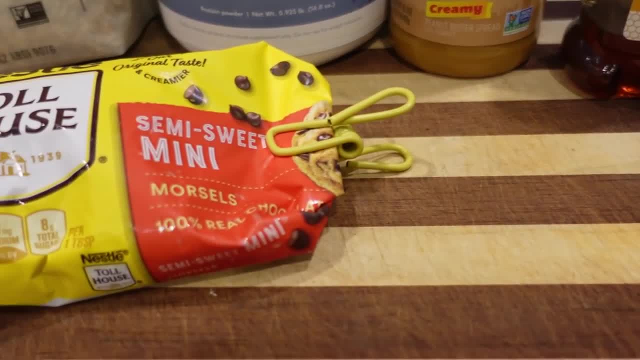 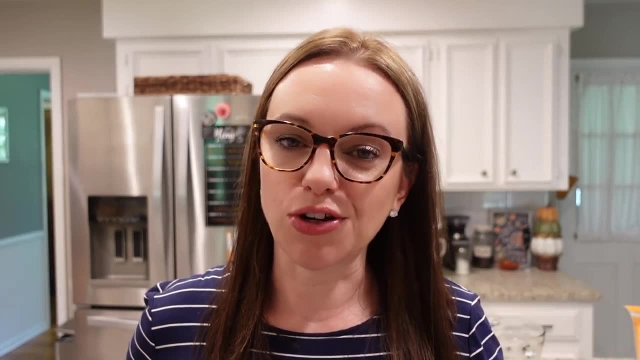 need them, And I just realized that three of the four recipes I've shared with you today have peanut butter in them, So I'm assuming that if you have a peanut allergy, or someone in your family does, there's other types of butter. I know there's sunflower butter. 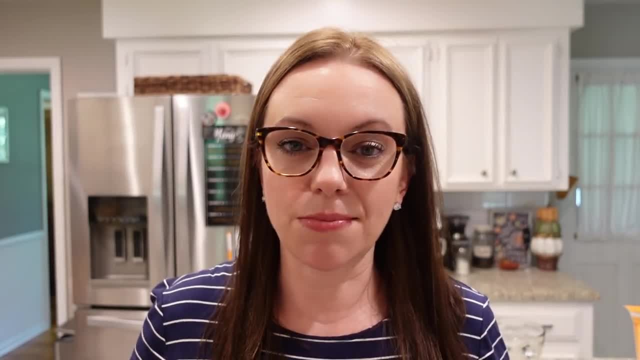 sunflower seed butter? I don't know, but hopefully you can adapt these to something that you like. So I'm going to show you how to make peanut butter. So I'm going to show you how to your family can use. And then I've got one other thing that I want to tell you about. 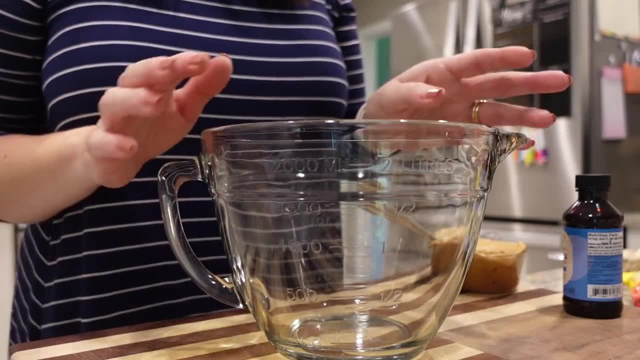 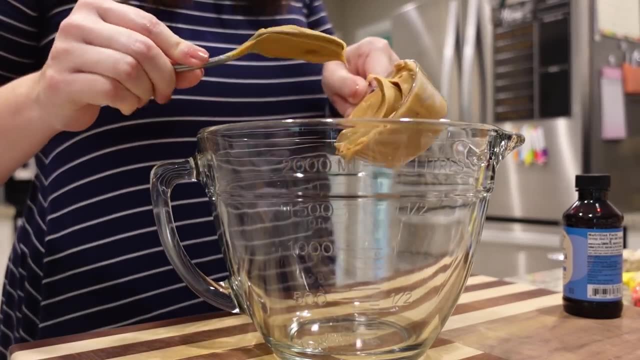 but I'll tell you that at the end of this recipe. Let's do it. Okay, this one's only going to take just a couple of minutes. The first thing we're going to do is just mix all of our ingredients together. I've got about three-fourths a cup of creamy peanut butter. I am cutting this recipe. 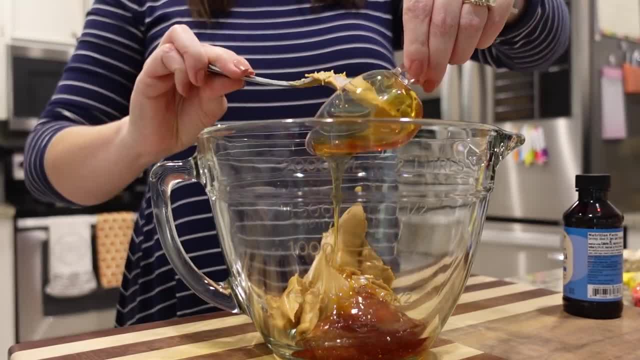 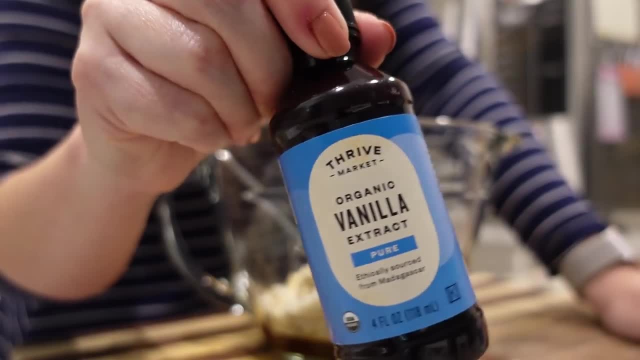 in half. The original recipe will be linked below. I've got about a fourth a cup of honey, two-thirds a cup of rolled oats. I've got some vanilla protein powder. I'm going to be using about a fourth a cup And I just realized I had this out and I didn't even need it out. 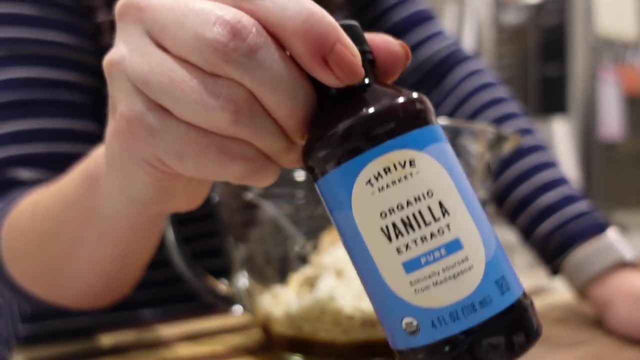 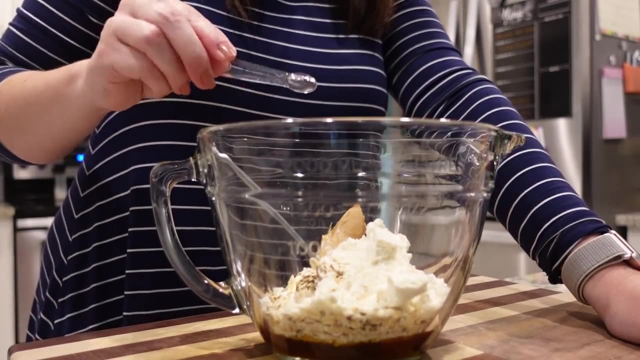 So yeah, we don't need vanilla. I grabbed this instead of the salt, So let me go grab the salt. When you saw this in the beginning, just forget. you saw this. I'm going to be adding just a tiny little pinch of salt, about a sixteenth of a teaspoon, because for the full recipe you need. 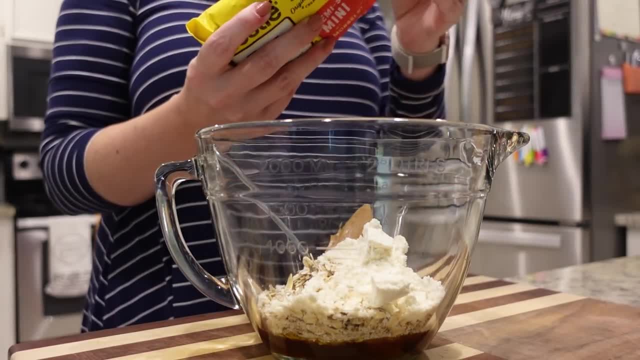 an eighth of a teaspoon. And lastly, I'm adding in about a fourth a cup of mini chocolate chips. Mine are semi-sweet, The recipe calls for dark. That's it. We're just going to mix all of this together. 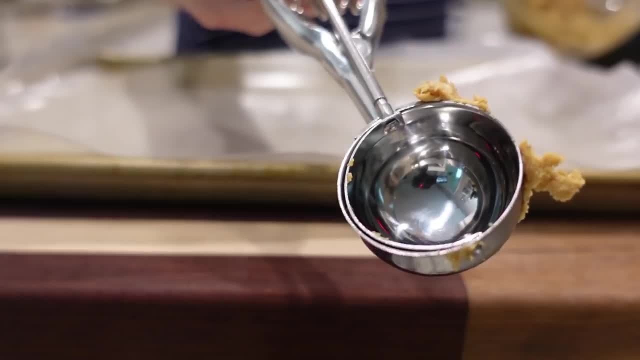 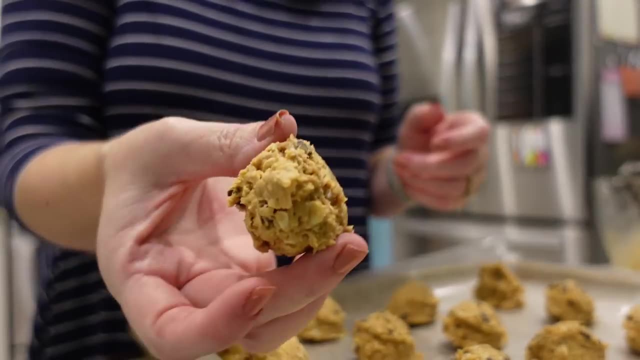 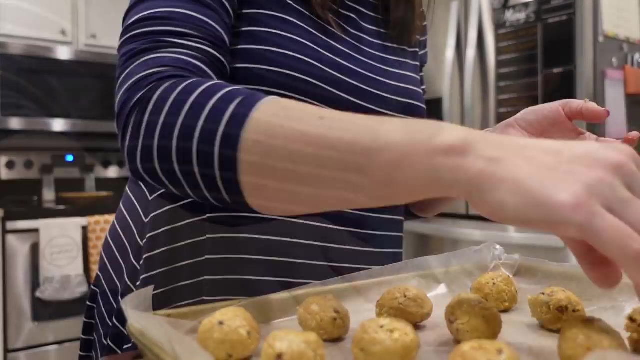 Now I've just got a baking sheet that I've covered with wax paper. I'm going to drop it by the spoonfuls here on this wax paper, and then I'll grab each one and roll them into a perfect little ball. Okay, these are just going to go in the fridge, just like this. for about an hour They should. 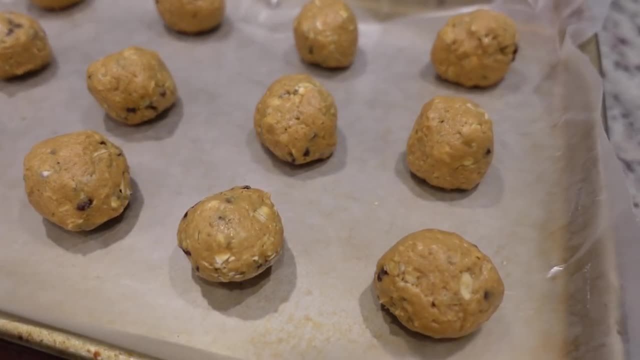 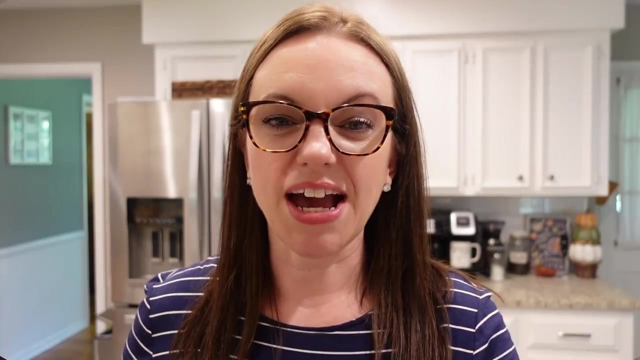 harden up after that, And then you can just put them in a gallon size bag and put them in the freezer just to have on hand for an hour. So that's how you make an afterschool snack that has plenty of protein. Okay, I just put them in the fridge, but I did taste the mixture and it's so, so good. So I give it two thumbs up. 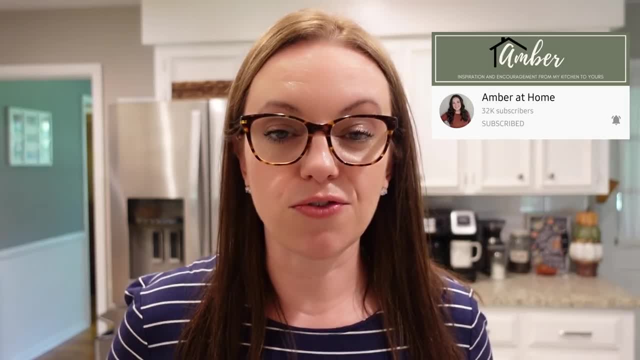 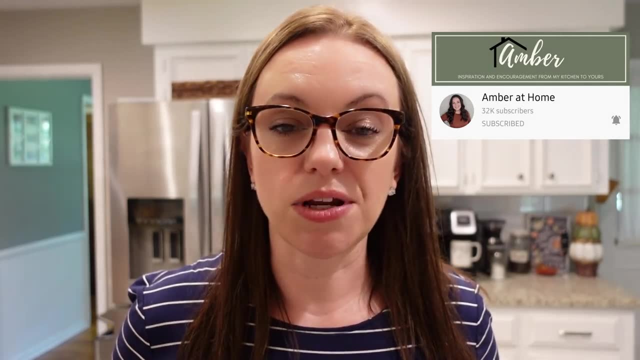 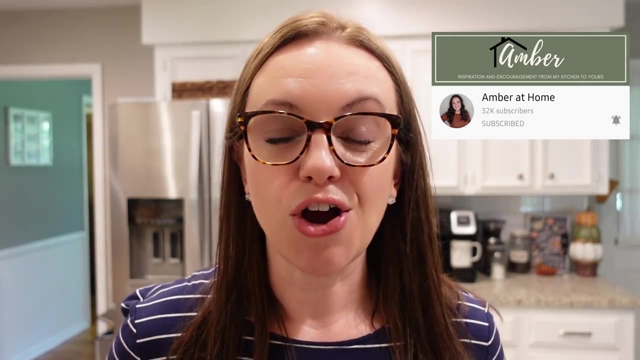 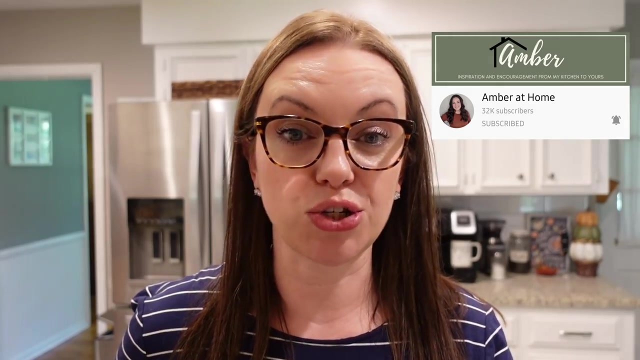 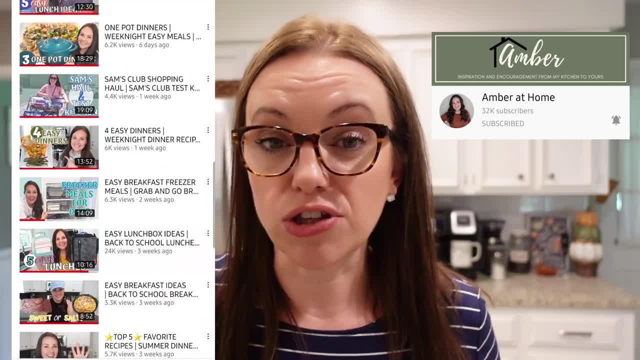 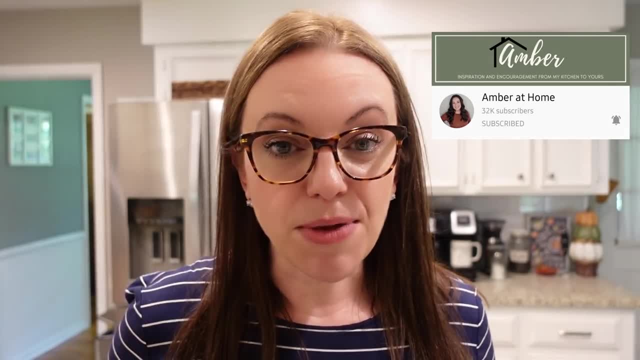 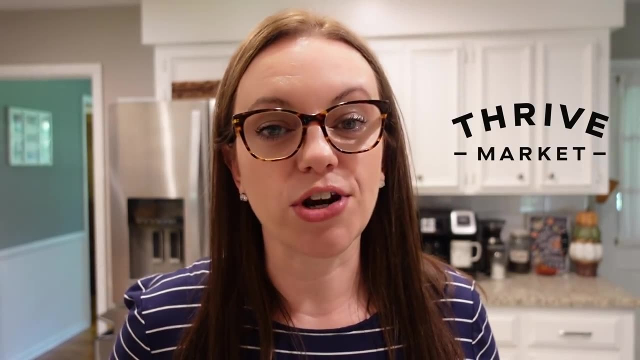 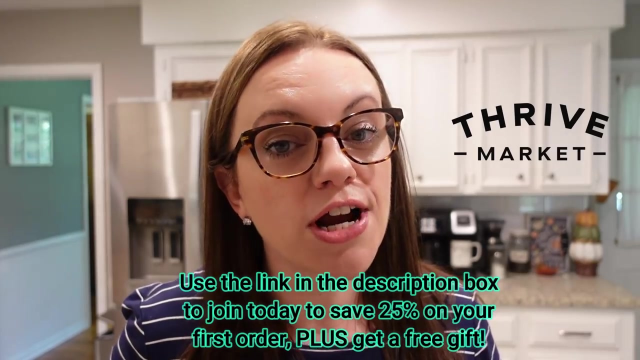 videos that I know a lot of people are enjoying. So if you're looking for lunch ideas in addition to snack ideas, you need to go check out her channel. She also does what's for dinners, just like I do. So if you like my channel, you're going to love her channel. Go over, watch the video, subscribe and tell her I sent you. And don't forget, if you are wanting to try Thrive Market, check my description box below, because if you join today, you're going to save 25% on your first order and you're going to get a free gift. Thanks again to Thrive Market for sponsoring today's video. I hope you all enjoyed it. 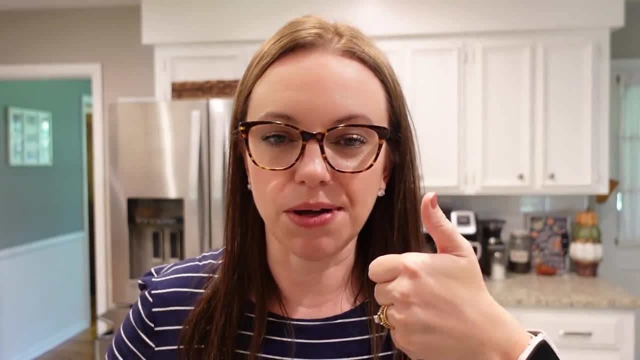 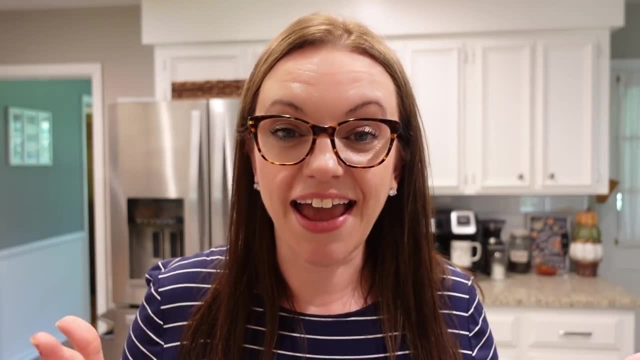 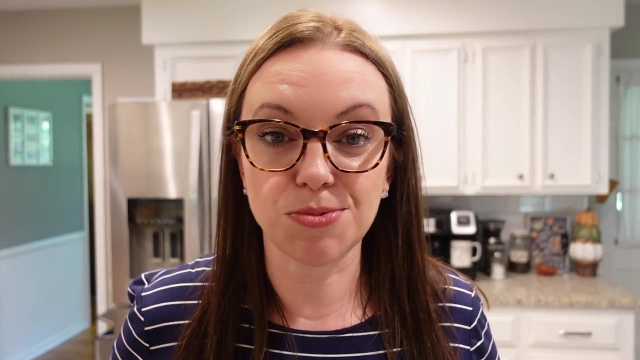 Don't forget to give me a thumbs up. You can only give one, but I wish you could give two. And if you made it to the end and you came over from Amber's channel- and this is your first time here- hi, I'm so glad you're here. I do content similar to this all of the time, So if you enjoyed this video, I would love for you to subscribe and stick around. Thank you all so much for watching. I hope you have a wonderful day and I'll see you back here soon. Bye.